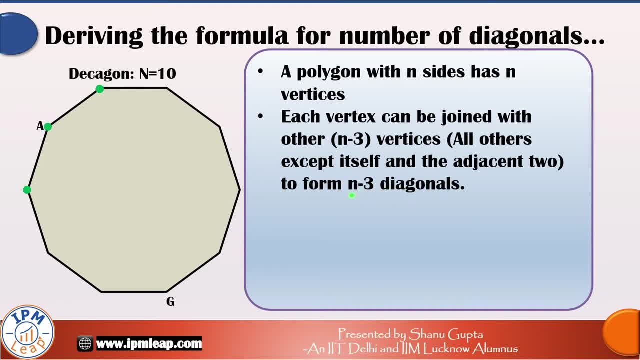 We will call the polygon of n with n-3 vertices. So this polygon of n will have exactly n vertices originating from any vertex. Let me illustrate this for the decagon on your screen. A decagon has 10 sides and 10 vertices, So let's suppose I select vertex A, the green dot, and try to join. 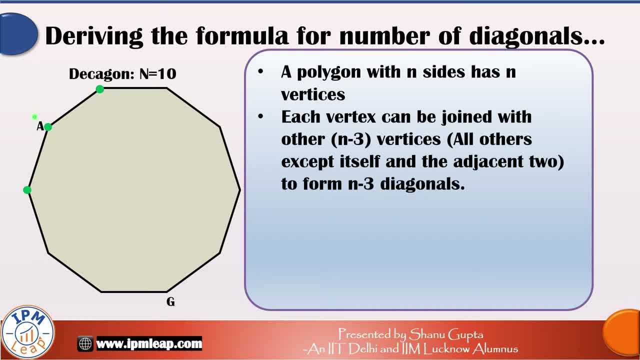 it to other vertices to form diagonals. So I will be able to join it to all other vertices in this decagon except itself and the adjacent two vertices shown by green dots. Out of 10 vertices, 10 minus 3, that is 7, can be joined with our selected vertex A and that forms 7 diagonals. 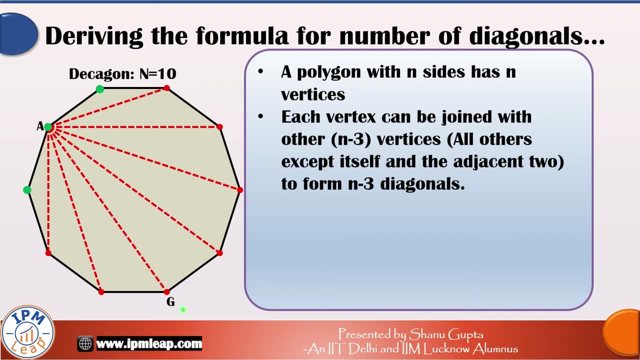 Similarly, it's easy to see that there will be 7 diagonals originating from each vertex. So let's take a count of these diagonals: 7 diagonals per vertex and 10 vertices in all, that makes 7 into 10, that is, 70 diagonals. But there is a catch here. 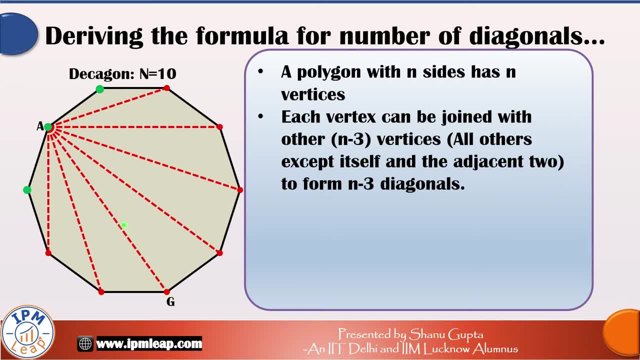 Each diagonal has 7 vertices in all, So let's take a count of these diagonals. diagonal gets counted twice in this scheme. For instance, if I take the diagonal AG, this diagonal gets counted when we were counting the diagonals originating from A and will. 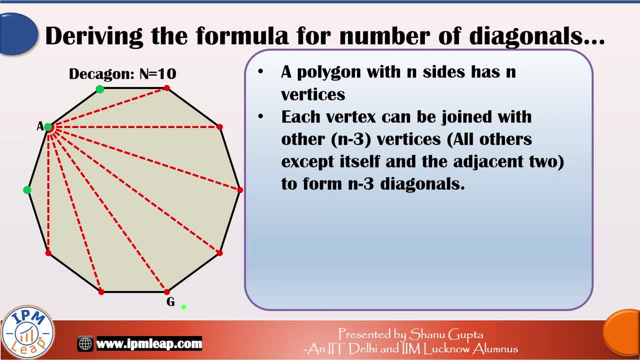 get counted again when we are counting the diagonals originating from vertex G. So all we need to do is divide this count 70 by 2 to get our actual number of diagonals. Therefore, a decagon will have 70 divided by 2, ie 35 diagonals. Let's extend this concept for 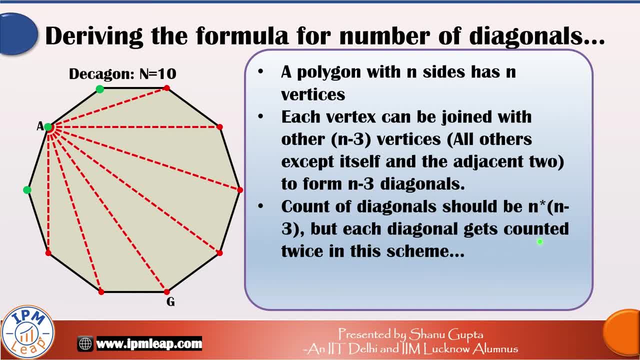 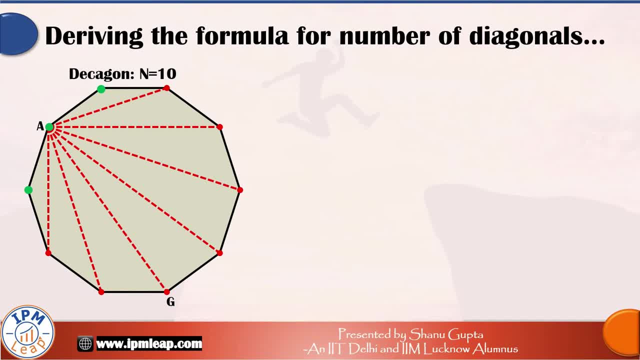 a polygon of n sides. The number of diagonals in a polygon of n sides will be n into n-3 divided by 2.. Now I am going to give you an alternate and much easier derivation of the same formula. It goes like this: Whenever we select any 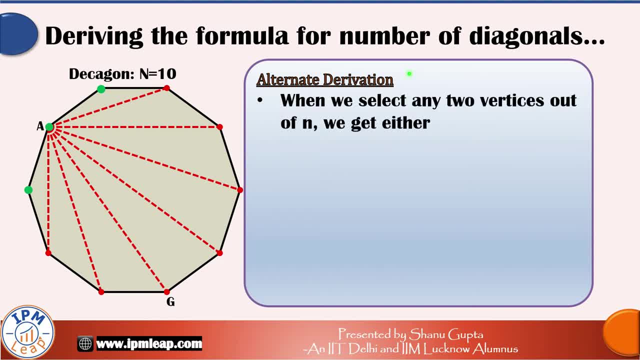 two vertices out of n, we get either a diagonal or a side of the polygon, Isn't it? So number of diagonals is simply equal to the number of ways of selecting two vertices out of n, minus the number of sides. Number of diagonals is equal to nC2, which is the number of ways of 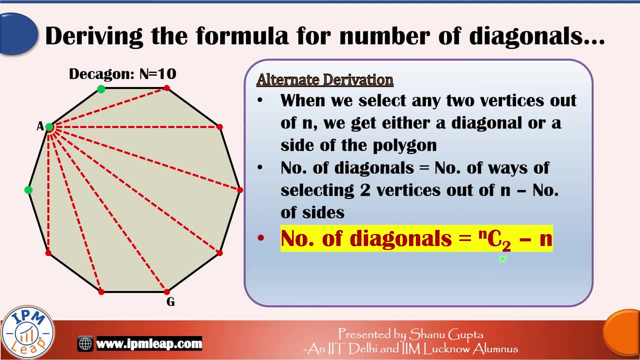 selecting two vertices out of n minus n, the number of sides. Once you master the concept of combinations, Let's see how this works. You will know that this formula for the number of diagonals simplifies to n into n minus 3 divided by 2.. 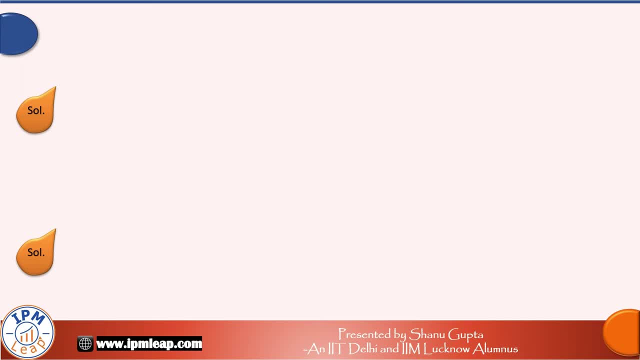 Finally, let's practice two questions on this concept. The first is: how many diagonals does a convex polygon with 11 sides have? So n is equal to 11. here, Number of Diagonals is equal to n into n-3 divided by 2.. So N. is 11,. we get 11 into 11 minus 3.. So n is also equal to 11 here. Let's see how this is done. So our frame looks like this. So our frame looks like this: We have only one diagonal. 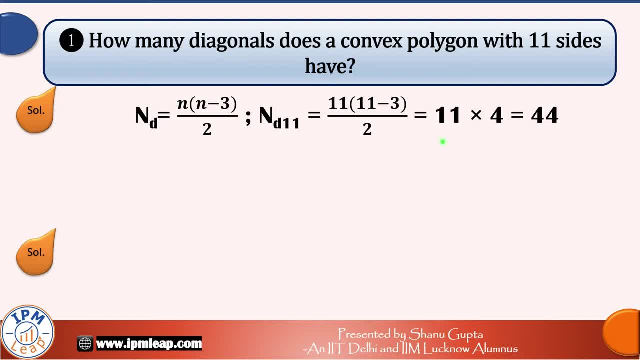 divided by 2. That is 11, into 4. 44 diagonals. So a polygon of 11 sides has 44 diagonals. The next question is: if a polygon has 65 diagonals, how many sides are there in the? 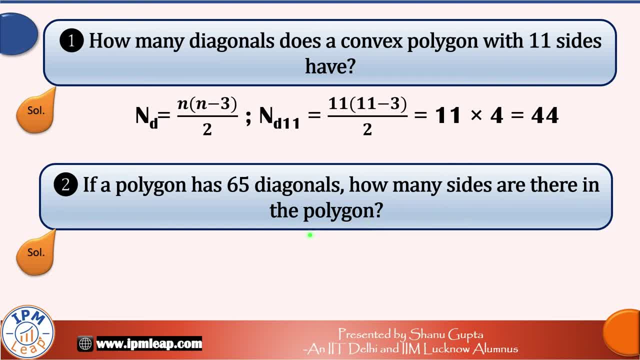 polygon. So number of diagonals in terms of sides is n into n minus 3 divided by 2.. That is given, and we have assumed that the polygon has n sides right, So number of diagonals is equal to 65. Multiply this equation with 2 on both sides. we get n into n minus 3 is. 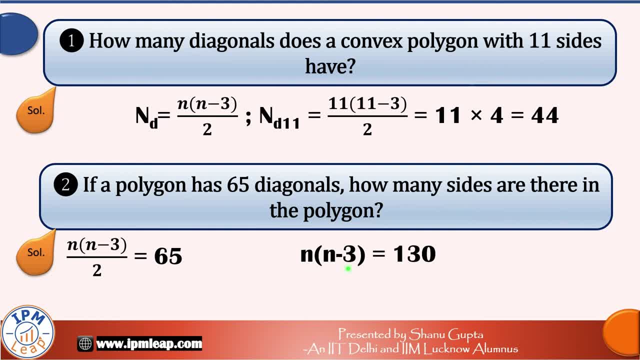 equal to 130.. Now, even though this equation is a quadratic equation, we can solve it by trial and error because, don't forget, n is a natural number. It stands for the number of diagonals right. So try writing the right hand side as a product of two factors of 130 which are close and differ. 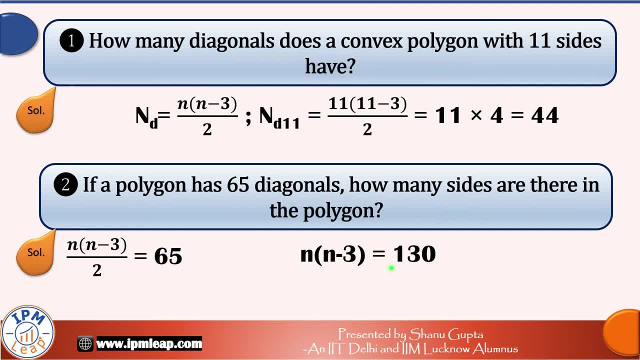 only by 2. So number of diagonals is equal to 65. So number of diagonals is equal to 1.. Because left hand side, we can see that n and n minus 3 differ by 3, right. So we know 130 can. 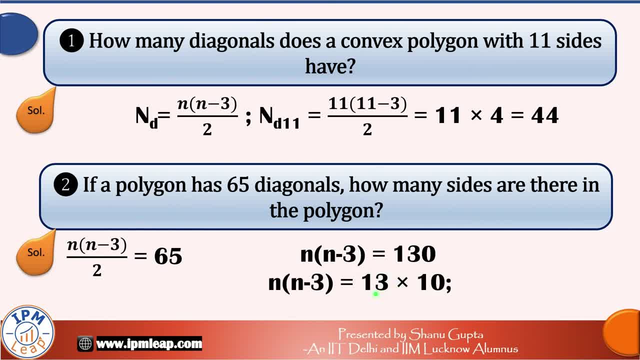 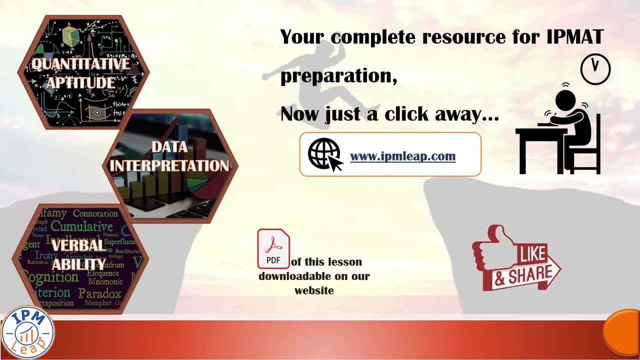 be written as 13 into 10. And therefore, comparing both sides of the equation, n is equal to 13.. Hope you enjoyed this maths lesson. Don't forget to press the like button if you did, and also press the bell icon next to subscribe to get notifications.